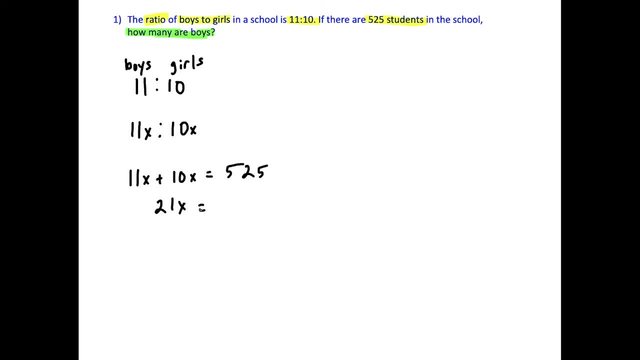 So then we just simplify here: We get 21x equals 525. And when you solve for x, divide by 21 on both sides- This is going to simplify, We're going to have So x equals and 525 divided by 21 is going to give us 25.. 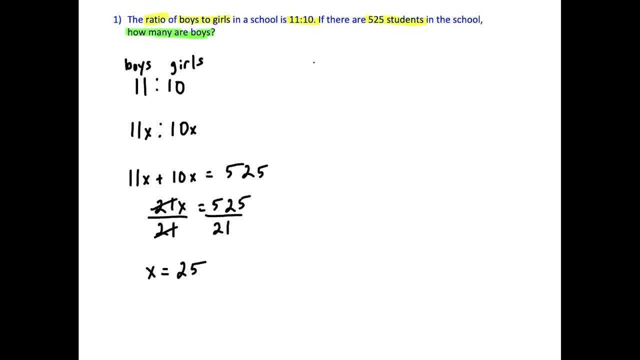 So x equals 25.. So then, how many boys are in the school? Well, the number of boys is 11 times 25.. And this is going to work out to 275.. So there are 275 boys. That's our final answer. 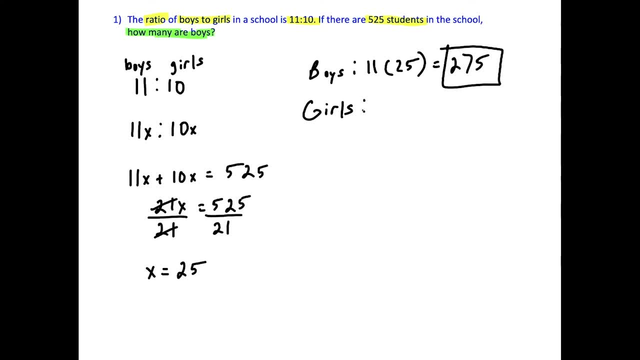 And the number, The number of girls, which isn't what we're told to find here, but it's good so we can check our work- that we find this as well- is 10 times x, which is 10 times 25, giving us 250. 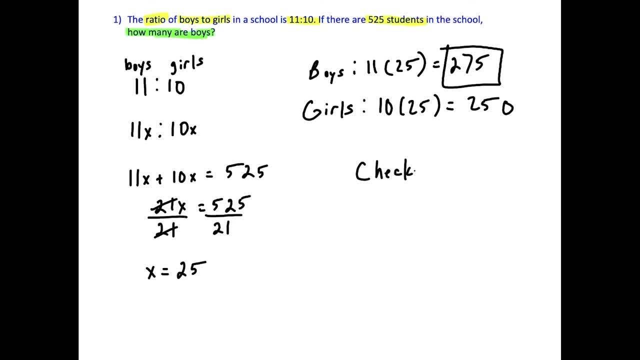 And now just to check, when we add these numbers together we should get 525.. So 275 plus 250 does in fact add up to 525.. And another thing to check here is to Compare these two numbers by division. divide the top and bottom by 25.. 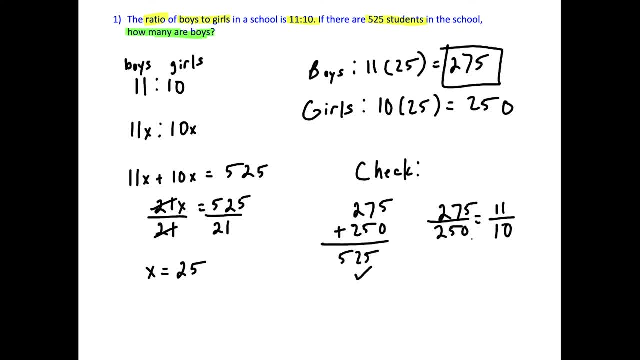 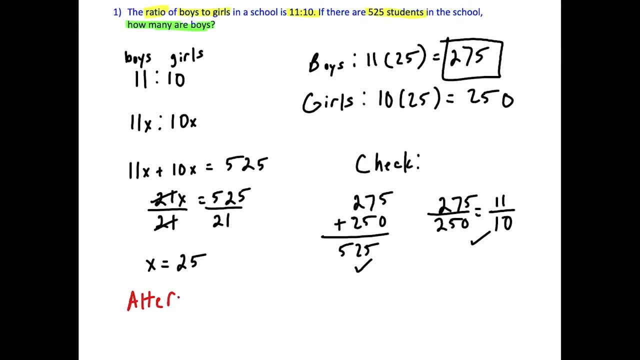 And this does simplify to 11 over 10.. So both of these things here check out. 275 is our solution to the first one. So an alternate method that we could use would be to use the concept of part over whole And just know if we're trying to find the number of boys. the number of boys. 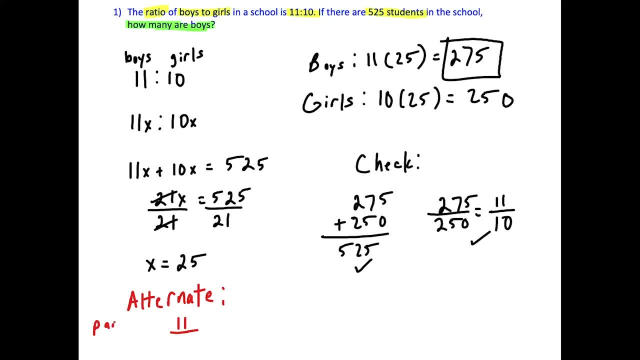 Well, that's, 11 is the part. So remember, the concept we're using is part over whole. And just know, if we're trying to find the number of boys, the number of boys, Well, that's, 11 is the part. 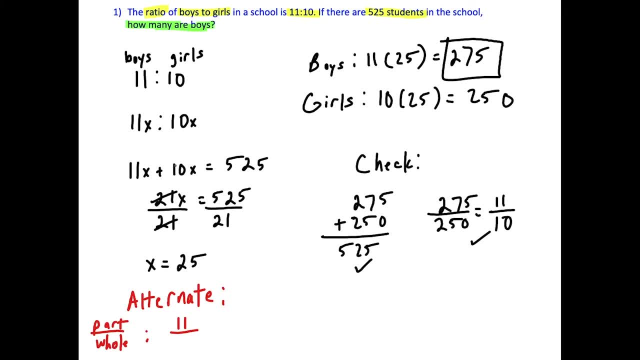 So remember, the concept we're using is part over whole, And when we use that concept here, the part is 11, and the whole would be 11 plus 10.. So for every 21 students, 11 are boys, Because we're told 11 boys for every 10 girls, that's 21 students in total. 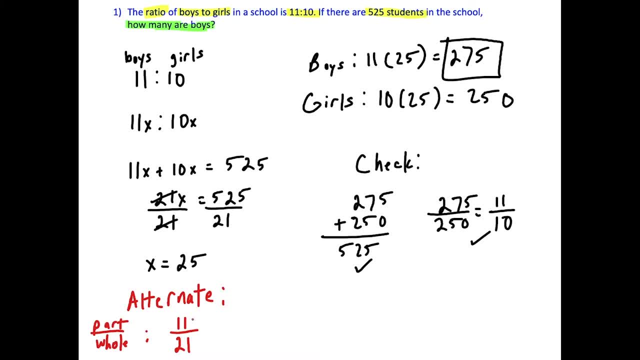 So out of the 21 students, 11 are boys. And if we multiply the part over whole by the total number of students- 525, that's going to tell us how many boys there are. And when we simplify this here, well, once again, 525 divided by 21 is 25.. 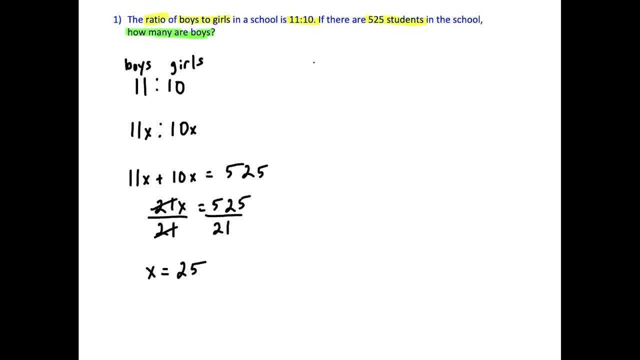 So x equals 25.. So then, how many boys are in the school? Well, the number of boys is 11 times 25.. And this is going to work out to 275.. So there are 275 boys. That's our final answer. 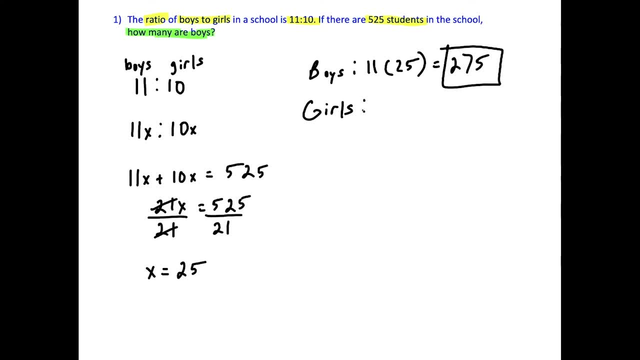 And the number, The number of girls, which isn't what we're told to find here, but it's good so we can check our work- that we find this as well- is 10 times x, which is 10 times 25, giving us 250. 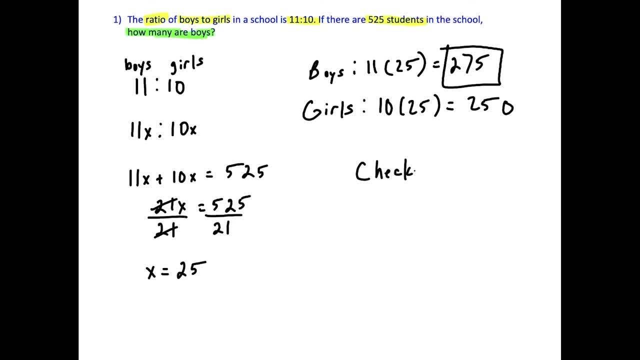 And now just to check, when we add these numbers together we should get 525.. So 275 plus 250 does in fact add up to 525.. And another thing to check here is to Compare these two numbers by division. divide the top and bottom by 25.. 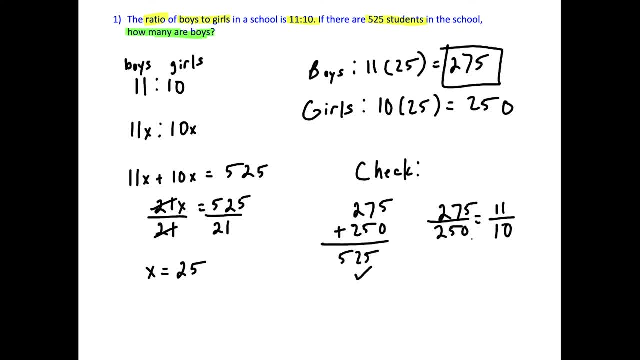 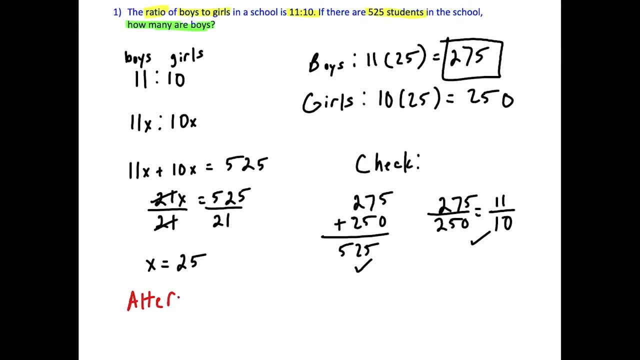 And this does simplify to 11 over 10.. So both of these things here check out. 275 is our solution to the first one. So an alternate method that we could use would be to use the concept of part over whole And just know if we're trying to find the number of boys. the number of boys. 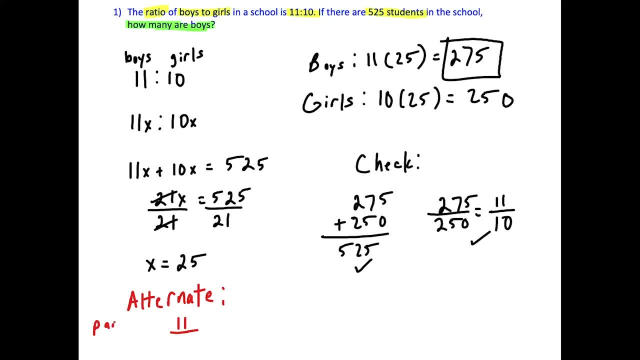 Well, that's, 11 is the part. So remember, the concept we're using is part over whole. And just know, if we're trying to find the number of boys, the number of boys, Well, that's, 11 is the part. So remember, the concept we're using is part over whole, And just know if we're trying to find the number of boys, the number of boys. Well, that's, 11 is the part, And just know if we're trying to find the number of boys, the number of boys. 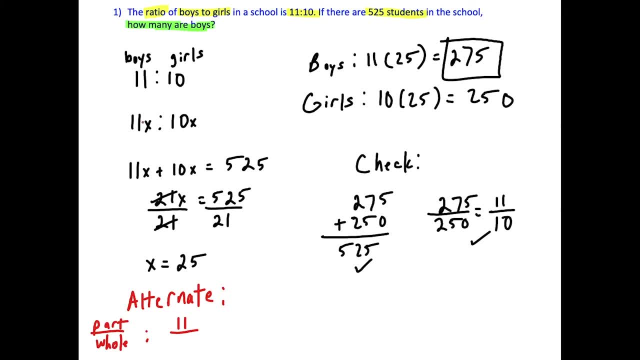 And when we use that concept here, the part is 11.. And the whole would be 11 plus 10.. So for every 21 students, 11 are boys, Because we're told 11 boys for every 10 girls. that's 21 students in total. 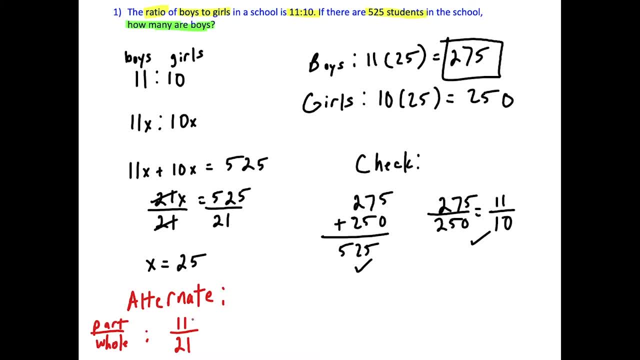 So out of the 21 students, 11 are boys. And if we multiply the part over whole by the total number of students- 525, that's going to tell us how many boys there are. And when we simplify this here, well, once again, 525 divided by 21 is 25.. 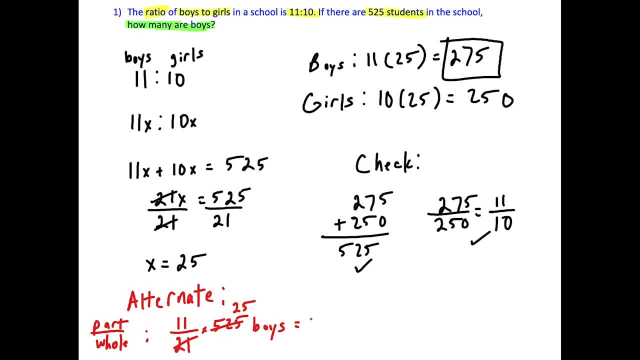 And when we multiply 11 times 25, we also get 275. So this is another method here is to write the part over whole and multiply it by the total number of students, And that'll tell you how many boys you have. 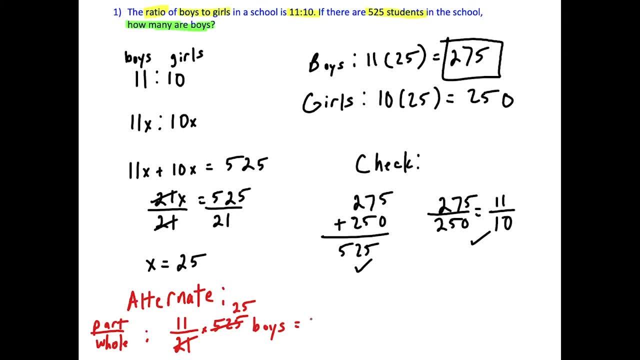 And when we multiply 11 times 25, we also get 275. So this is another method here is to write the part over whole and multiply it by the total number of students, and that'll tell you how many boys you have. 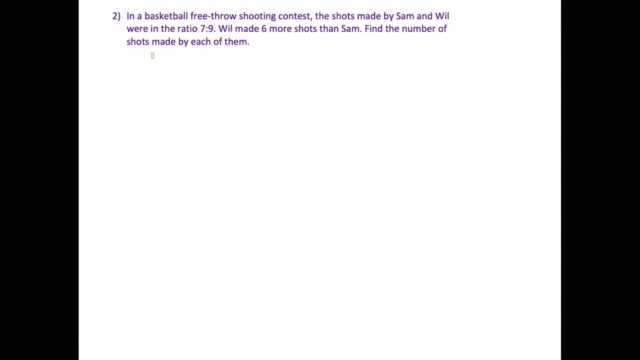 All right for this last question. here we have a basketball free throw shooting contest And the two participants are Sam and Will, And they're telling us that for every seven shots that Sam made, Will made nine. So this is the ratio of their shots: seven to nine. 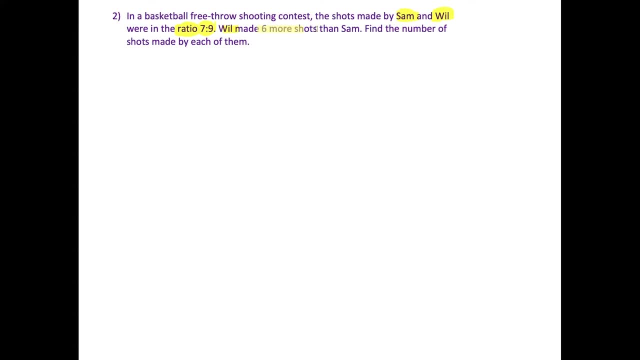 And we're also told that Will made six more shots than Sam, And we want to find the number of shots made by each of them. So think really carefully about this here. So the ratio is the first thing we could write down: seven to nine. 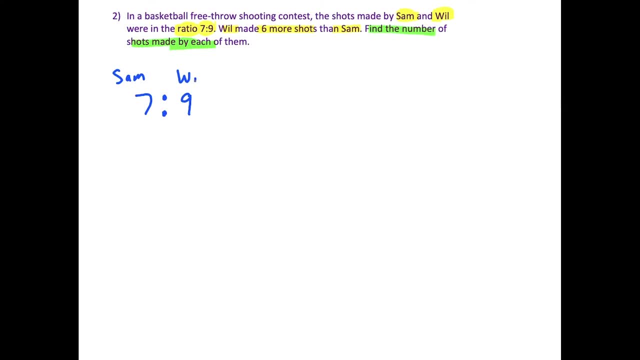 And this is comparing Sam, And this is comparing Sam to Will. But what they're telling us is that Will made six more shots than Sam. So if Sam made x shots, so this is like the number of shots that he made in. well then Will is going to be x plus six because he made six more, so that's plus six. 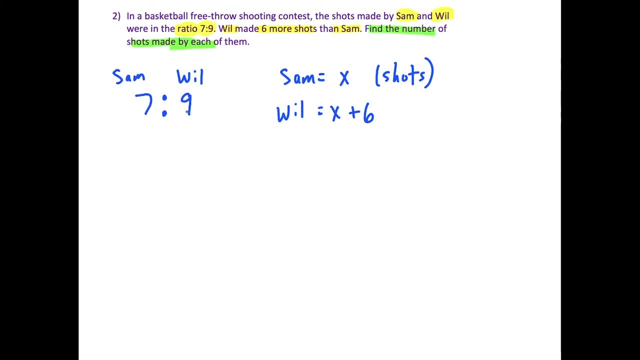 So then we combine all this information, The ratio. So the ratio of Sam to Will is seven over nine. But remember, this top part is for Sam, The bottom part is for Will. And we're also told that if Sam made x shots, Will made six more, made x plus six. 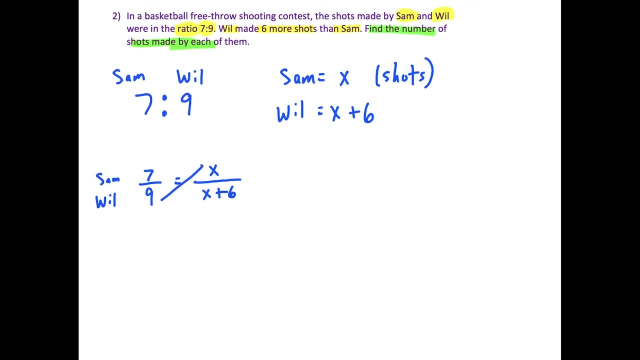 So to solve this equation here, let's cross multiply. We're going to multiply nine times x, And that's equal to seven times x plus six. But just make sure to throw the x plus six in parentheses. We have to distribute here. 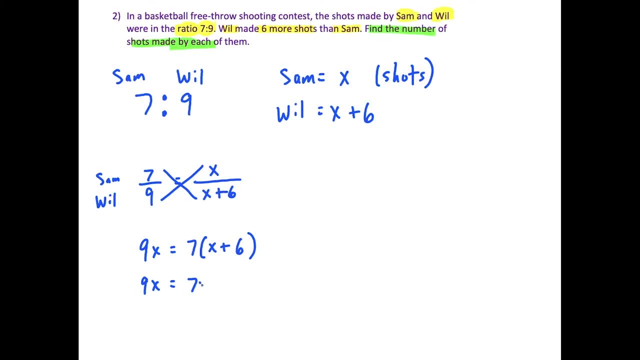 So then let's work this out. This is nine x equals seven x plus 42.. Remember, just make sure to multiply seven by x and positive six. Now we subtract seven x on both sides And I'll write the result over here. 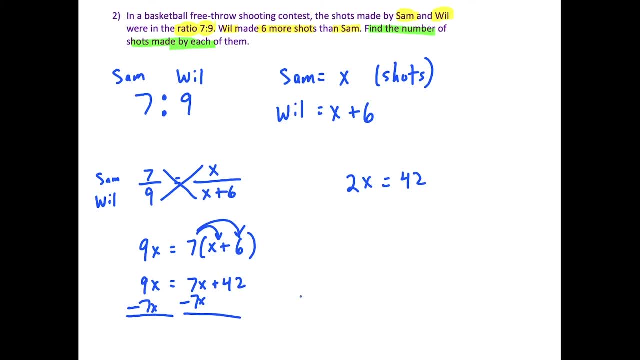 We have: two x equals 42. So that results from before is going here And then divide both sides by two, All right, So that's two x, And we're told that x equals 21. So if we write all this out, this tells us that Sam made 21 shots. 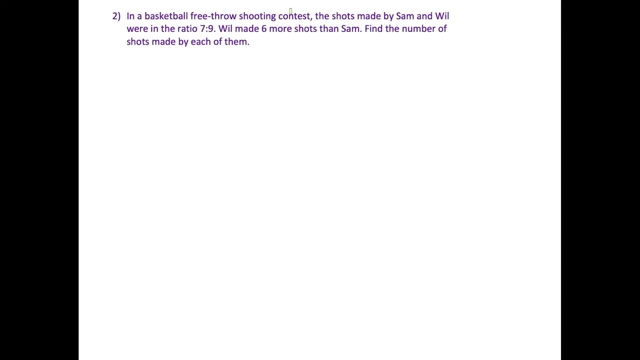 All right for this last question. here we have a basketball free throw shooting contest And the two participants are Sam and Will, And they're telling us that for every seven shots that Sam made, Will made nine. So this is the ratio of their shots: seven to nine. 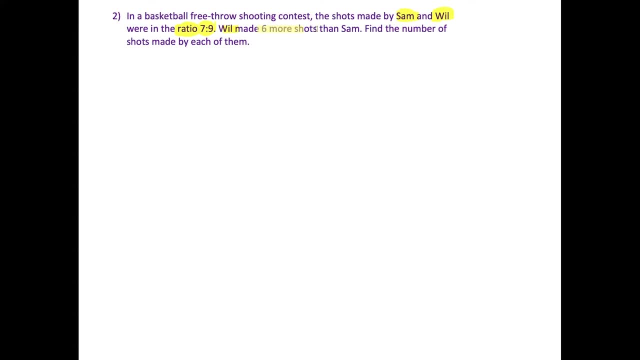 And we're also told that Will made six more shots than Sam, And we want to find the number of shots made by each of them. So think really carefully about this here. So the ratio is the first thing we could write down: seven to nine. 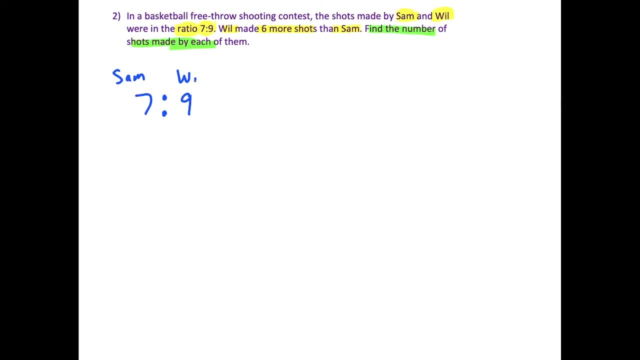 And this is comparing Sam And this is comparing Will. But what they're telling us is that Will made six more shots than Sam. So if Sam made X shots, so this is like the number of shots that he made in- well then Will is going to be X plus six. 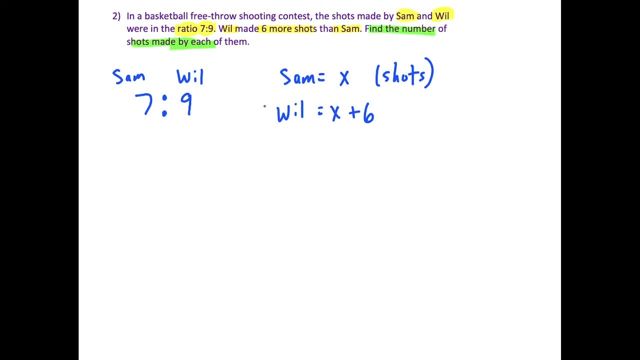 Because he made six more. so that's plus six. So then we combine all this information, The ratio Sam to Will is 7 over 9. but remember, this top part is for Sam, the bottom part is for Will and we're also told that if Sam made X shots, Will made 6 more made. 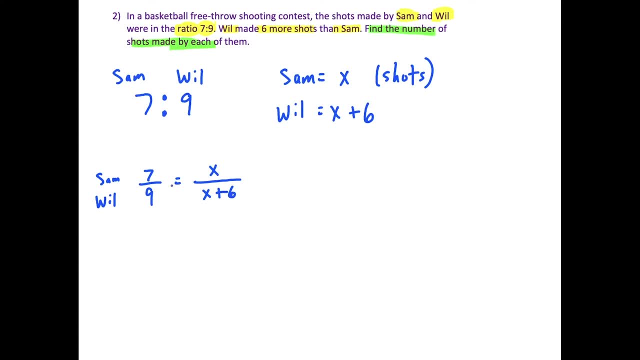 X plus 6. so to solve this equation here, let's cross multiply. we're going to multiply 9 times X, and that's equal to 7 times X plus 6, but just make sure to throw the X plus 6 in parentheses. we have to distribute here. so then let's 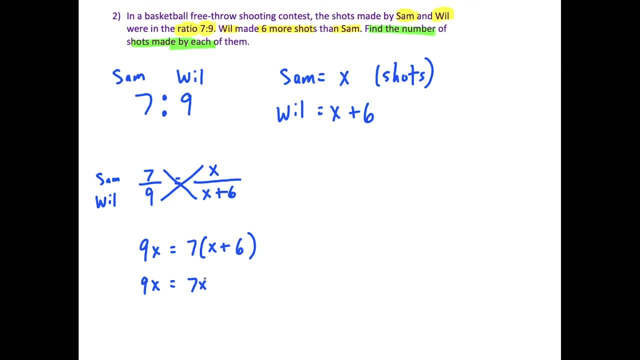 work this out. this is 9 X equals 7 X plus 42. remember, just make sure to multiply 7 by X and positive 6. now we subtract 7 X on both sides and I'll write the result over here. we have 2 X equals 42, so that results from before is: 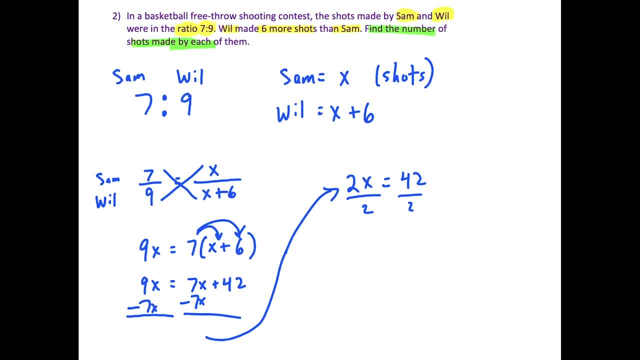 going here and then divide both sides by 2 and we're told that X equals 21. so if we write all this out, this tells us that Sam made 21 shots and Will made 6 more than that, and 21 plus 6 is 27. now the